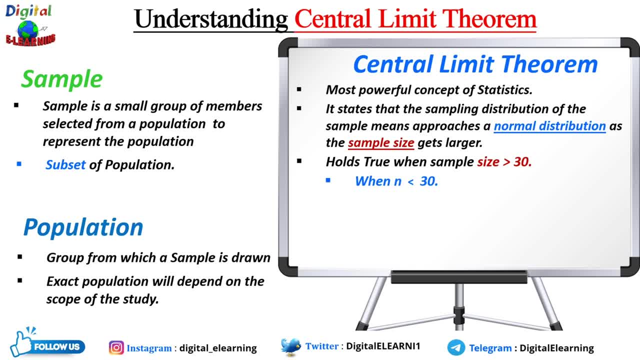 of population. Therefore the sampling distribution will only be normal if population distribution is also normal. But when n is greater than 30 or equal to ready central limit theorem applies here. The sampling distribution will approximately follow a normal distribution Because n is greater after 30.. maker. or similarly, If the sample distribution is similar to 30, central limit theorem applies here- The sampling distribution will shout only positive fieldsże. So the grateful distribution will only include edges. The upstream distribution will also need normal. Similarly enough n será mistaken to infinity, though communityこんな was esper 물. 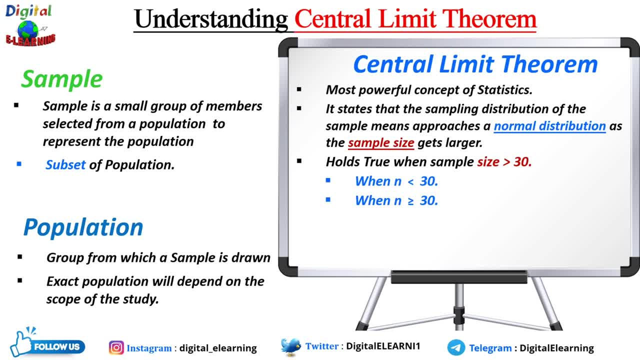 distribution. so, in short, if your sample size is less than 30, your central limit theorem will not apply and the sampling distribution will follow what we have for distribution for a population, and when it is greater than 30 it will follow a normal distribution, irrespective of what is the distribution. 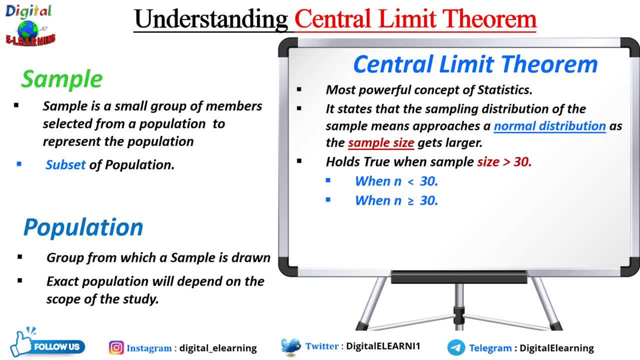 that we have for population. an essential component of central limit theorem is that average of your sample mean will be there as population mean. in other words, add up the mean of all your samples, find the average of it and then the average will be your actual population mean. similarly, if you find the average of all, 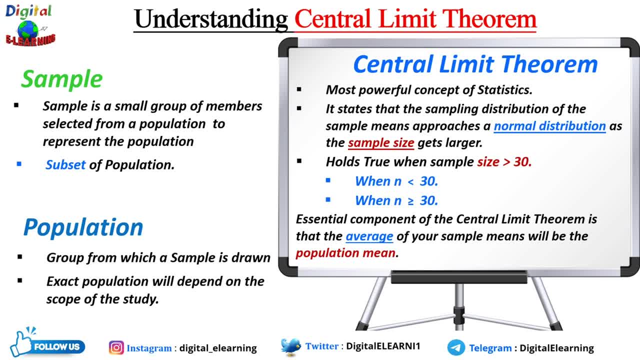 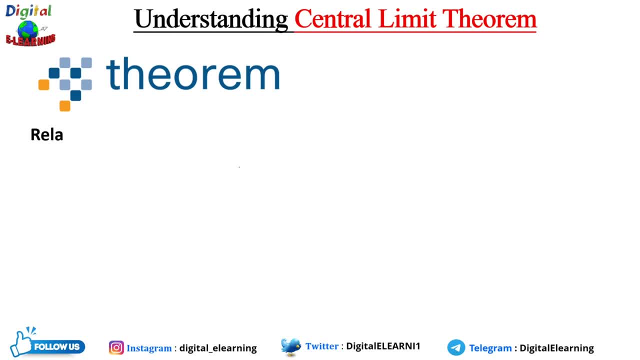 the standard deviations. in your sample you will find the actual standard deviation for your population. so, as per the theorem, the relationship between the shape of population distribution and the shape of sampling distribution of a mean is known as the central limit theorem. the significance of a central limit theorem is that it 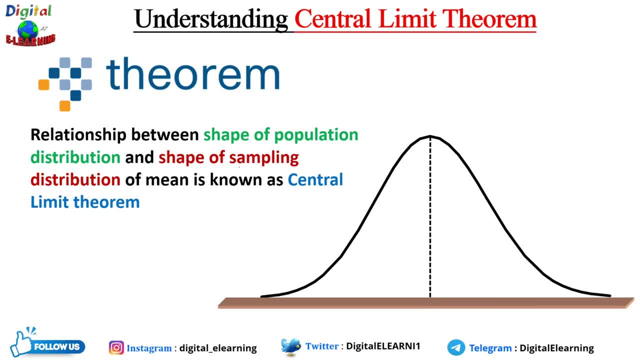 permit us to use the sample statistics to make the inference about population parameters without knowing anything about the shape of the frequency distribution of that population. let's take an example of a fair rolling dice. the more time each person roll a dice, more likely the shape of distribution of a mean tends to look like a normally distributed graph. 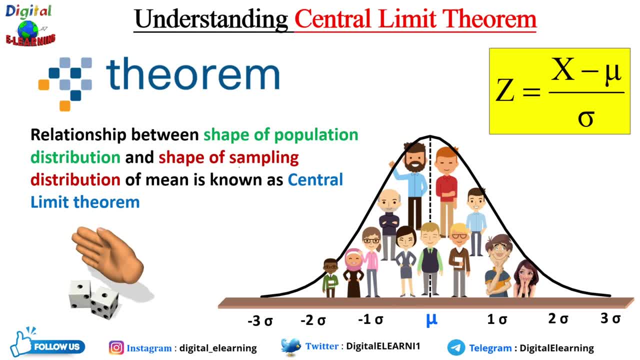 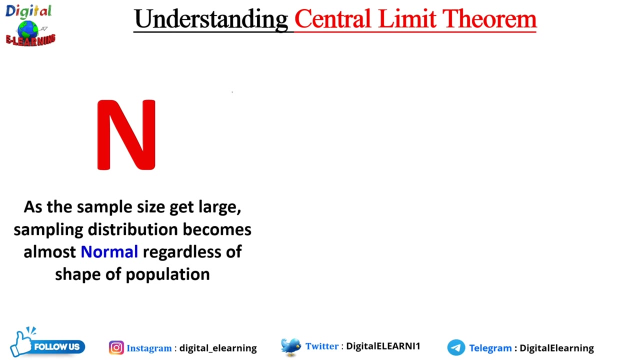 so central limit theorem is applicable for sufficiently large sample size. as I just discussed previously. when n is greater than 30, the formula is Z equal to X minus mu by Sigma. this is the formula for that we use for central limit theorem and the sample size, so as the sample size gets large, the sampling 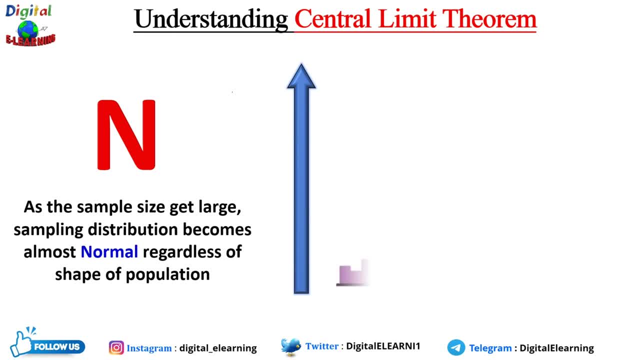 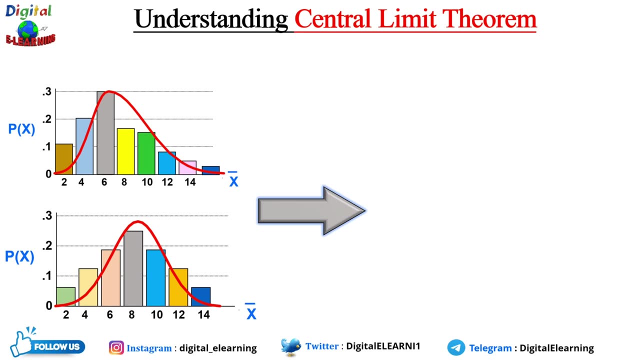 distribution becomes almost normal, regardless of the shape of the population. so if your population distribution is flat, bimodal, unimodal Poisson distribution and will follow any kind of distribution, your end result would be if you take a sample from that population and that will always be a normal. 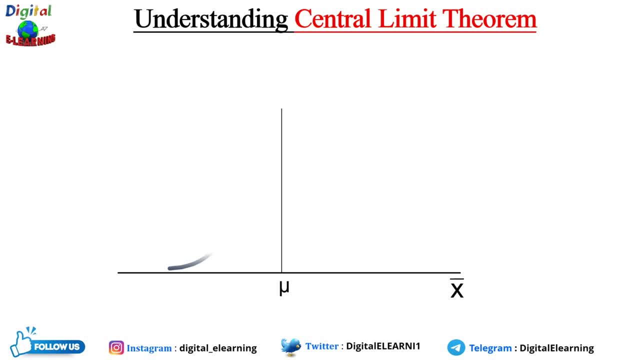 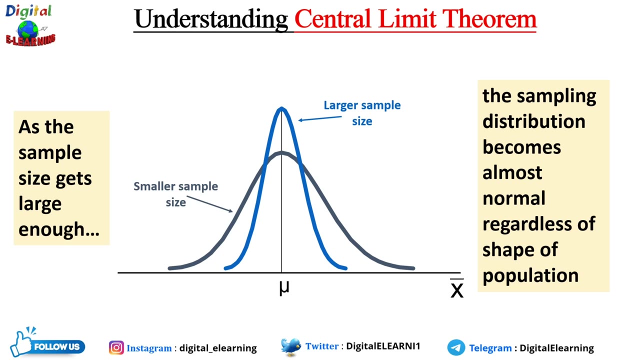 distribution. so if you take the same graph where you have a smaller sample size, as you go on increasing the larger sample size, as a sample size gets large enough, the sampling distribution becomes almost normal, regardless of the shape of the population's. that is how explained through graphically here. let's take an 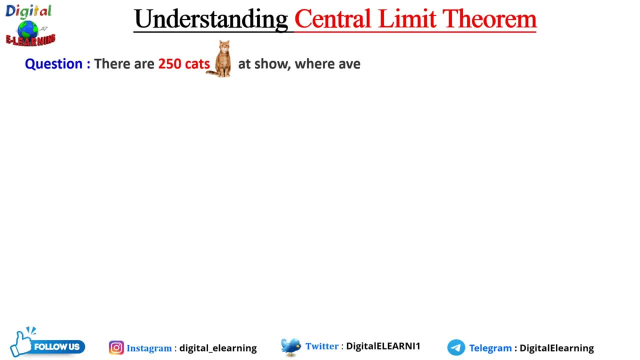 example, to understand this concept, there are 250 cats and to show where the average weight of cat is 12 kg, we standardize it for Anguilla to see the average weight of cat is 12 kg. we standardize it for Anguilla to see the. 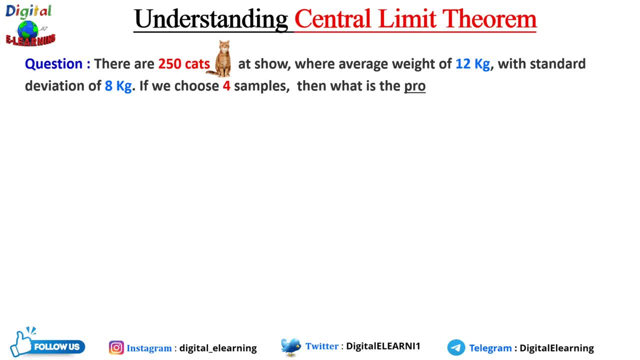 average weight of cat is 12 kg. we standardize it for Anguilla to see the with standard deviation of 8 kg. now if we choose four samples, and what is the probability that the average weight of cat is greater than 10 kg and less than? 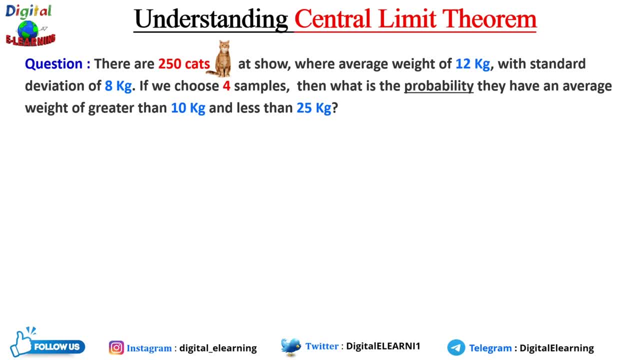 25 kg. this is the problem setting that we have in our hand now. mean of the population mu is 12 kg. that is given in the statement. standard deviation is 8 kg. it is also given in the statement. we have four samples and equal to four. we 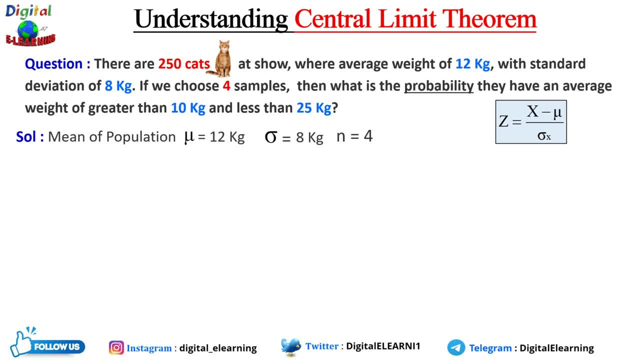 apply the standard limit theorem, formula Z equal to X minus mu by Sigma X, where mu denotes the population mean, Sigma denotes the population standard deviation, mu, X denotes the sample mean, Sigma X denotes the sample standard deviation and N denotes the sample of size. now we are given Sigma X, which is 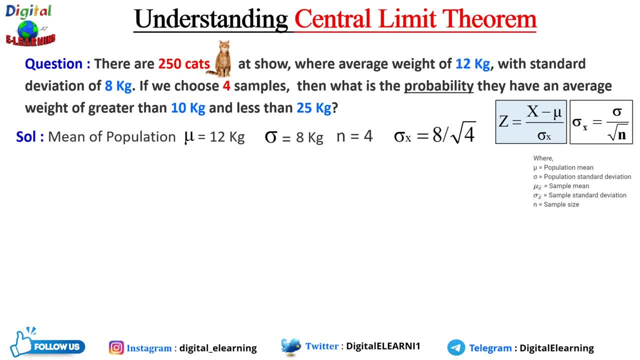 an under root of Sigma by under root of root of n. so we got Sigma standard division, which is given as 8 divided by under root of n and as 4. so we apply the normal curve here. we'll apply the limits 12 as mean and 10 and 25 as the upper. 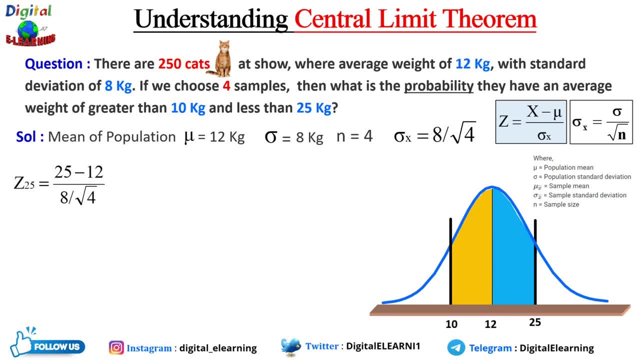 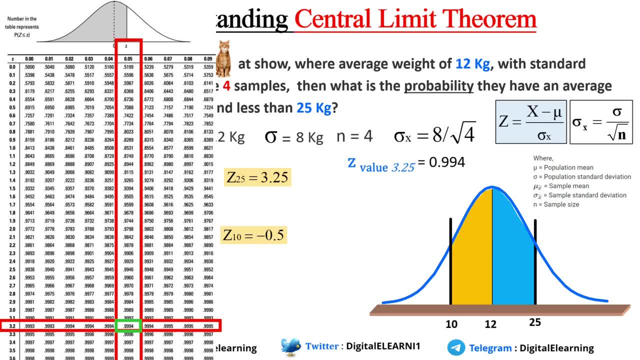 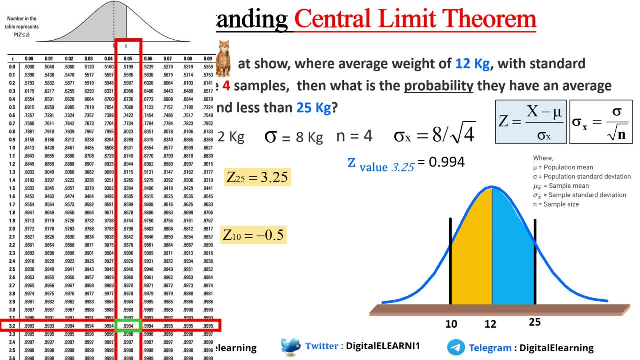 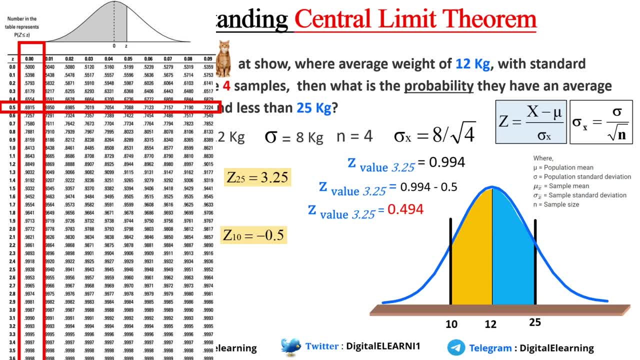 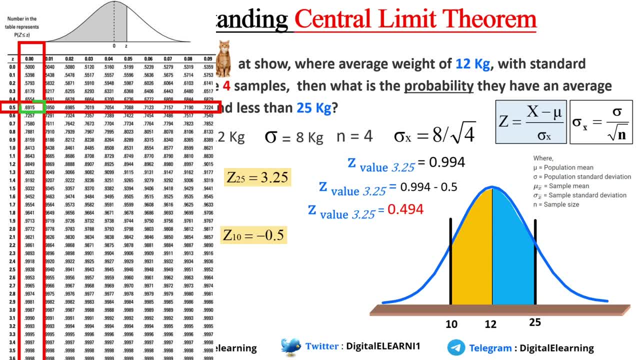 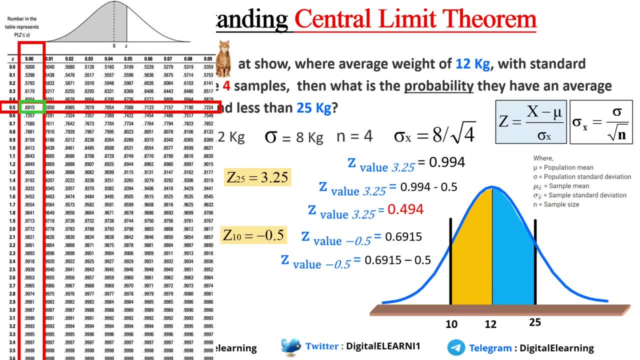 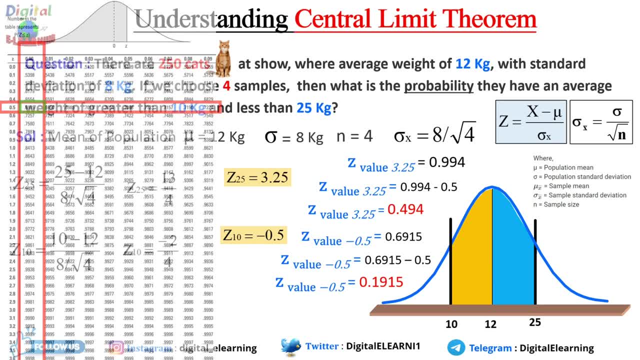 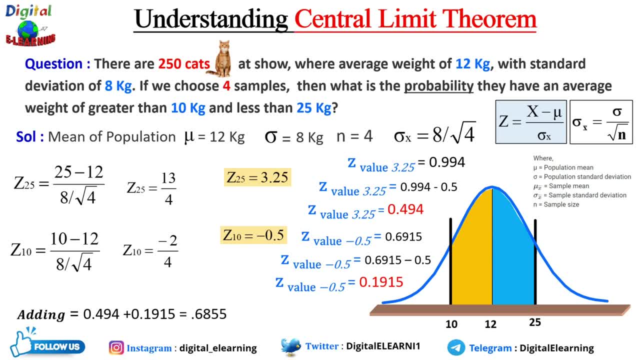 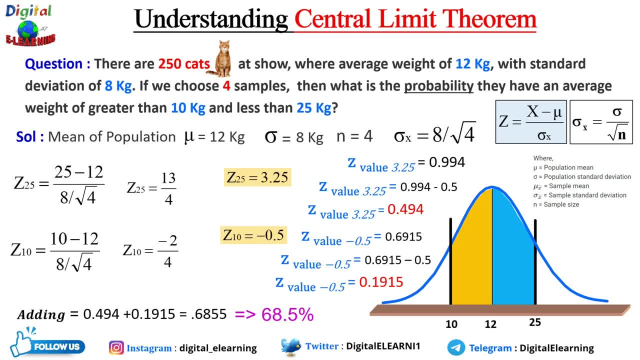 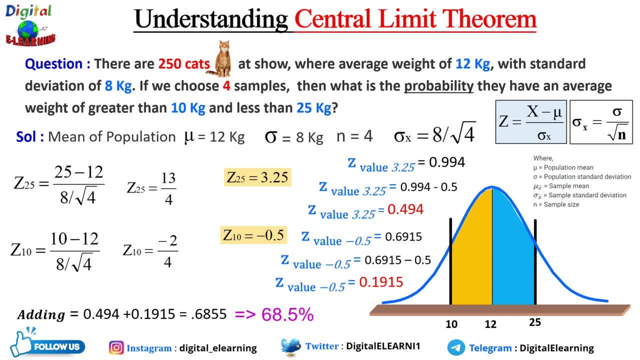 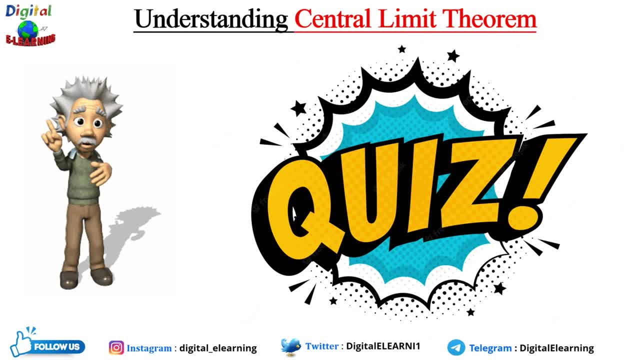 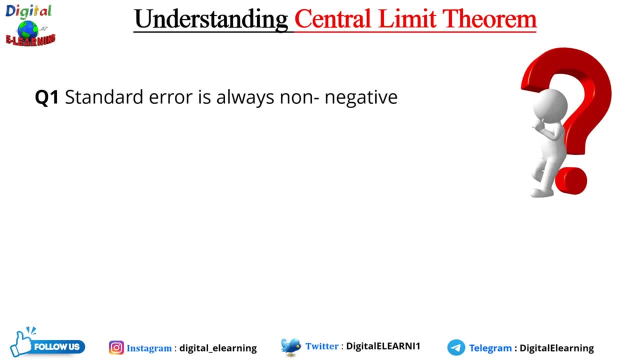 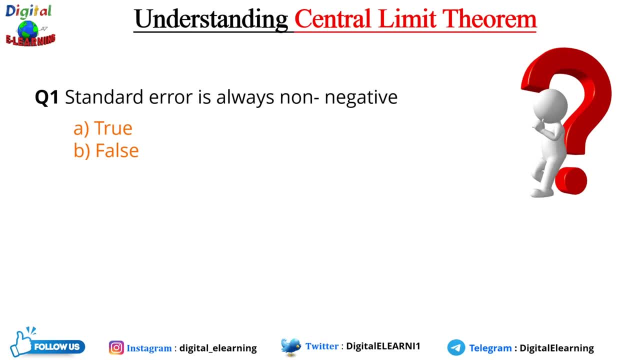 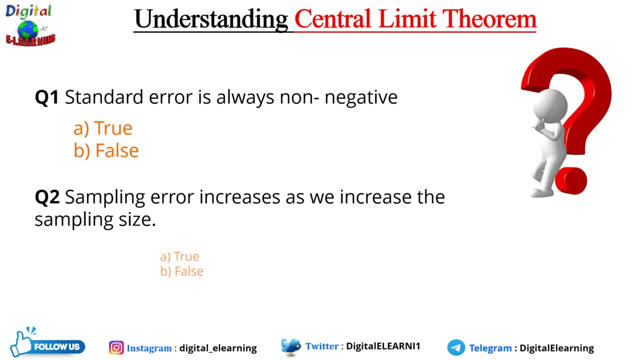